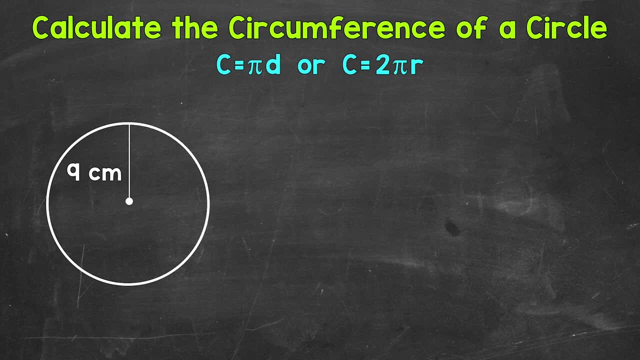 the formula. that includes the radius. And one more thing to keep in mind before jumping into our example, and that is pi. Pi is the same for all circles. It's a constant. Pi is the ratio of a circle to a circle. So if you're using the formula, circumference equals 2 pi r, so 2 pi r. 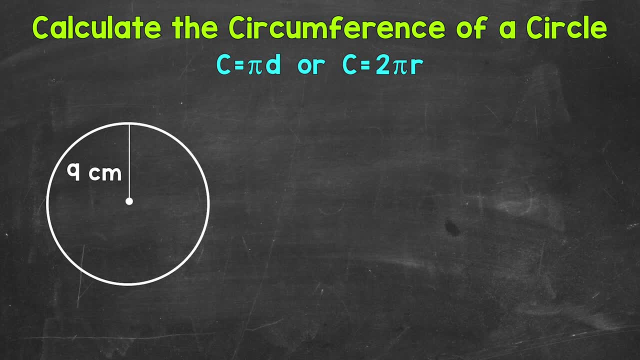 you're going to have a circle circumference to its diameter, So it's the circumference of a circle divided by its diameter. Let's jump into our example where we have a circle with a given radius of 9 centimeters. Now the first thing I'm going to do is write out our formula and we're 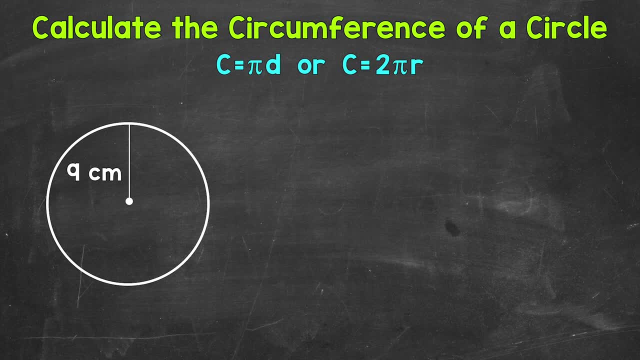 going to use. circumference equals 2 pi r, so 2 times pi times r. And we're using that formula since we are given the radius, So circumference equals 2 pi r. Now we can plug in the radius, So circumference equals 2 times pi. 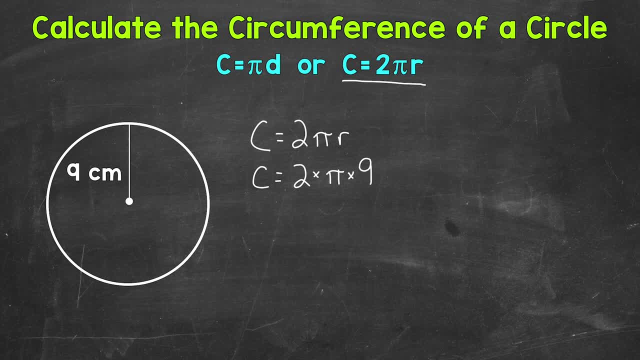 times the radius of 9 centimeters. Once we have that 9 plugged in for our radius, we can do 2 times 9, which is 18.. And for our next step, we can write that, as circumference equals 2 pi r, And we're going to use circumference equals 2 pi r, so circumference equals 2 pi r. 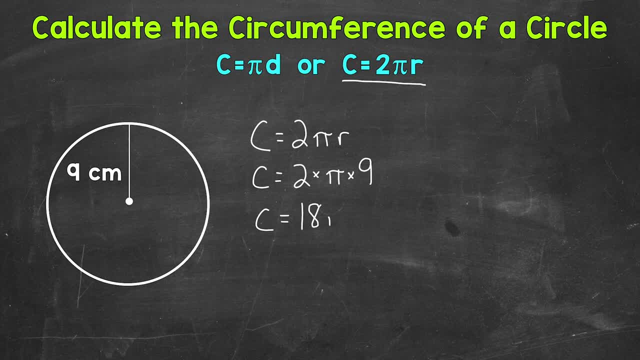 And we're going to use. circumference equals 18 pi r, So we put our number in front of the pi symbol. Now, this is one way to write the circumference, And this is called writing it in terms of pi, meaning we can write our number in front of the pi symbol and put our unit of measure. 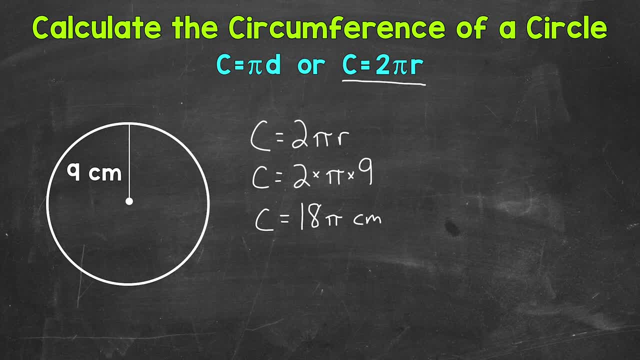 which is centimeters. So circumference equals 18 pi and again our unit of measure, centimeters. This is called writing it in terms of pi. Another way we can do this is to write our circumference in decimal form using an approximate value of pi, since pi is irrational And we're going to use 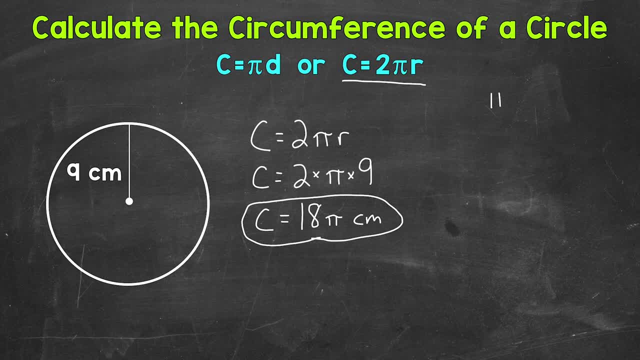 3.14. So we are going to use: pi is approximately 3.14. So that squiggly equal sign that means an approximate value rather than an approximate value. So we're going to use 3.14. And we're going to use: 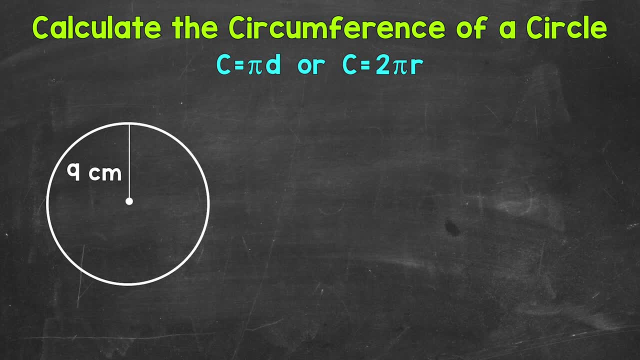 you're going to have a circle circumference to its diameter, So it's the circumference of a circle divided by its diameter. Let's jump into our example where we have a circle with a given radius of 9 centimeters. Now the first thing I'm going to do is write out our formula and we're 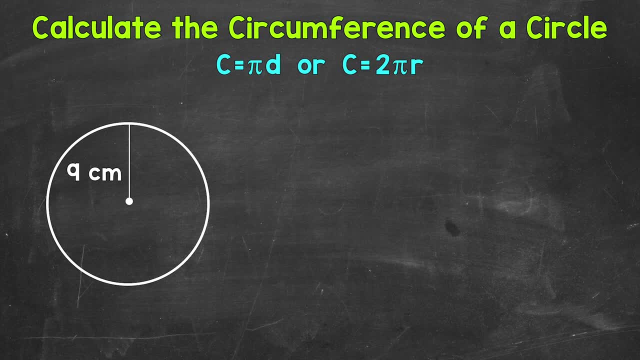 going to use. circumference equals 2 pi r, so 2 times pi times r. And we're using that formula since we are given the radius, So circumference equals 2 pi r. Now we can plug in the radius, So circumference equals 2 times pi. 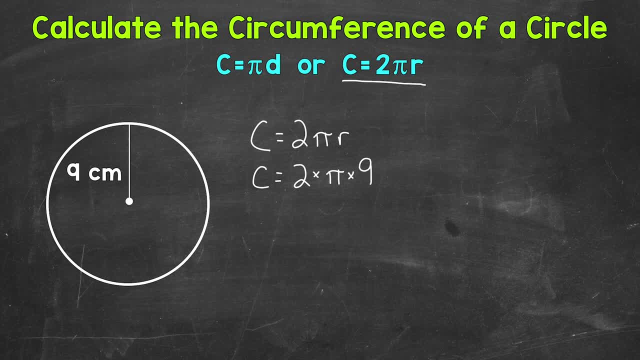 times the radius of 9 centimeters. Once we have that 9 plugged in for our radius, we can do 2 times 9, which is 18.. And for our next step, we can write that, as circumference equals 2 pi r, And we're going to use circumference equals 2 pi r, so circumference equals 2 pi r. 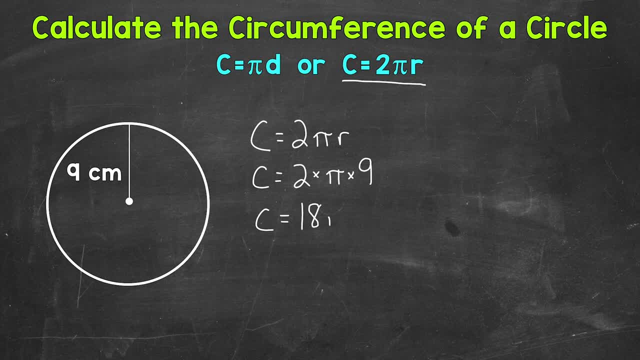 And we're going to use. circumference equals 18 pi r, So we put our number in front of the pi symbol. Now, this is one way to write the circumference, And this is called writing it in terms of pi, meaning we can write our number in front of the pi symbol and put our unit of measure. 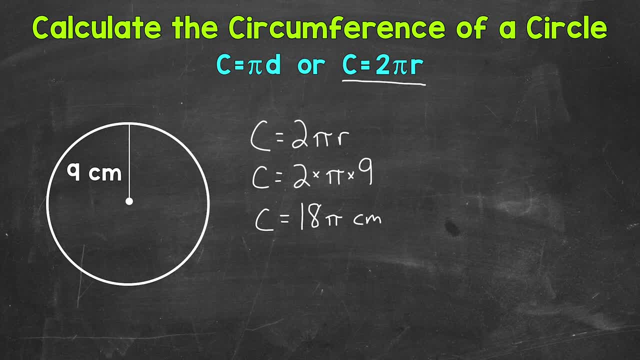 which is centimeters. So circumference equals 18 pi and again our unit of measure, centimeters. This is called writing it in terms of pi. Another way we can do this is to write our circumference in decimal form using an approximate value of pi, since pi is irrational And we're going to use 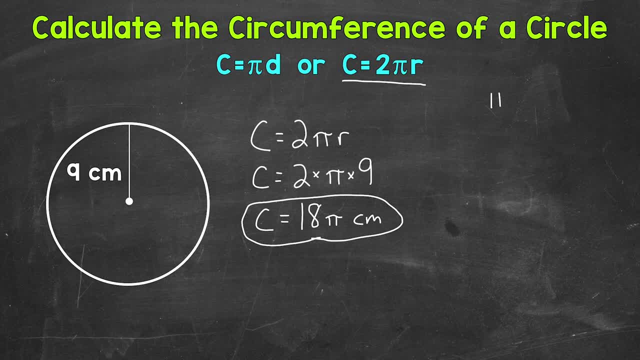 3.14. So we are going to use: pi is approximately 3.14. So that squiggly equal sign that means an approximate value rather than an approximate value. So we're going to use 3.14. And we're going to use: 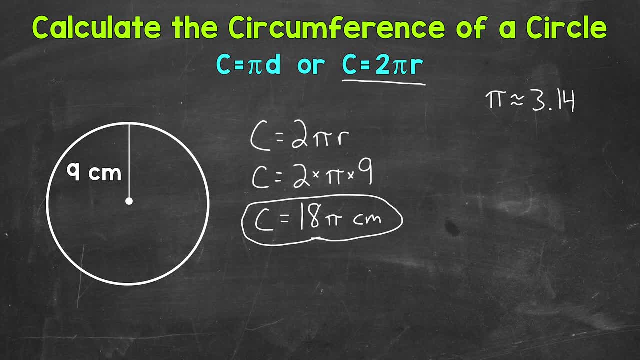 an equal sign, which means an exact value. So we can write out our formula: Circumference equals 2 pi r, And then we will plug in: So circumference is approximately. I'll use that approximate symbol because we are using an approximate value of pi, So 2 times 3.14 times our radius.